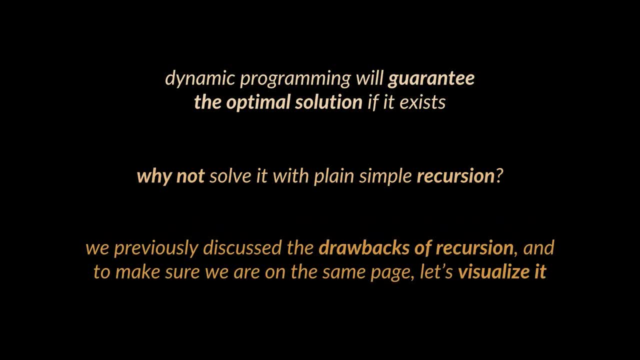 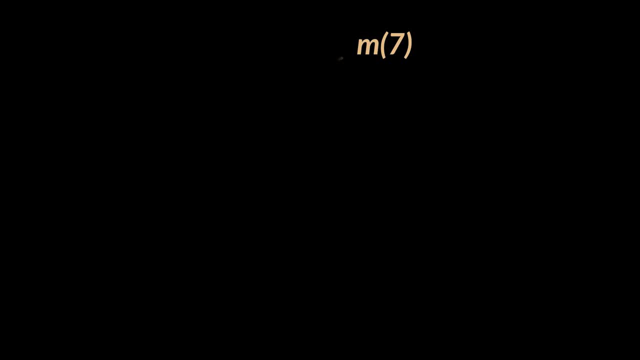 of recursion and to make sure we are on the same page, let's visualize it. You see, solving this problem is basically calling a recursive method. let's call it m and provide it with the target value 7.. Now, after this, we have 4 choices. we either picked the $1 coin and 6 remain, or we picked 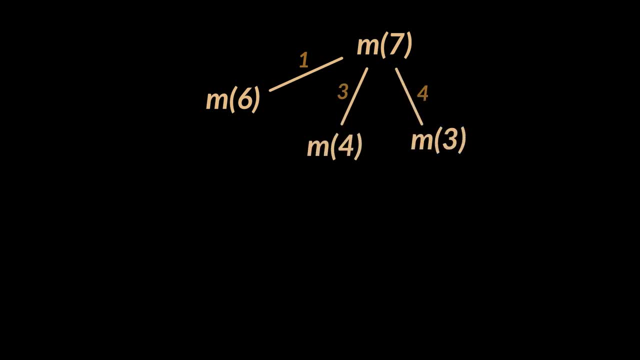 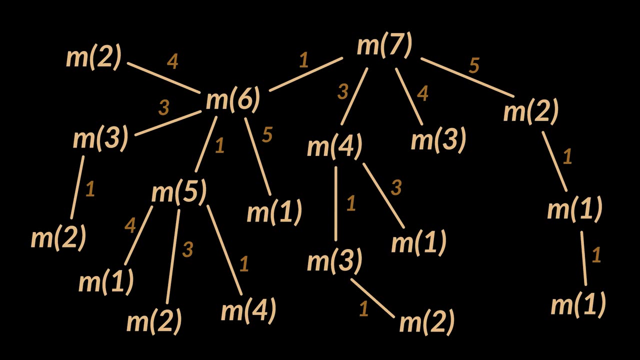 the $3 coin and 4 remain, or we picked the $4 coin and 3 remain, or we picked the $5 coin and 2 remain. This logic will keep on going until we find the solution, meaning until the amount we are providing to the recursive call is 0, right. 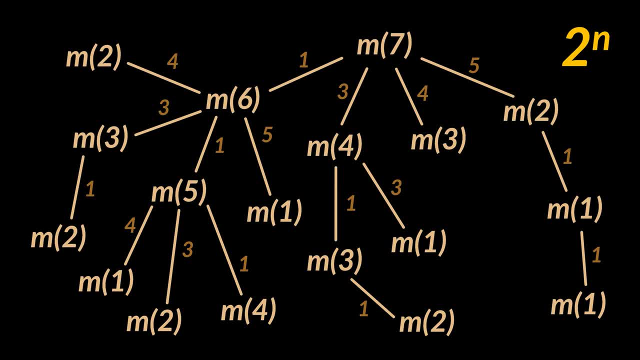 Well, the complexity of the tree, you see, is 2 to the power n, because we have overlapping sub-problems. We are calling this method with the same arguments more than once, and that is exactly what dynamic programming is about. It's about remembering the history and storing the values we previously retrieved so we can. 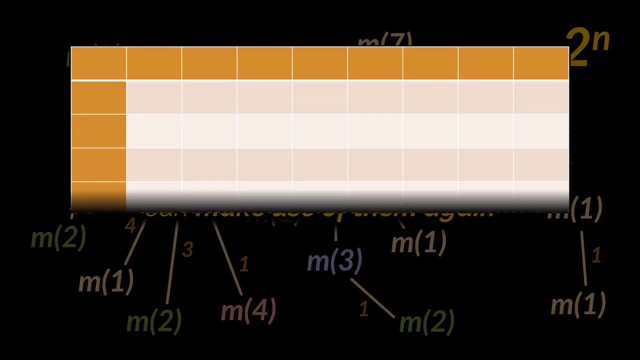 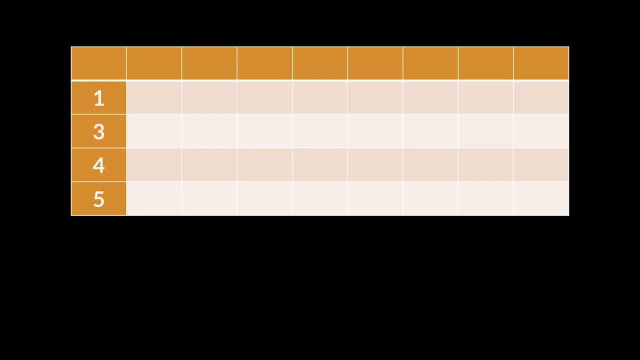 make use of them again. So let's go ahead and draw a 2D table. On the y-axis, we are going to list the coins we have, and on the x-axis, we are going to divide the problem into sub-problems and 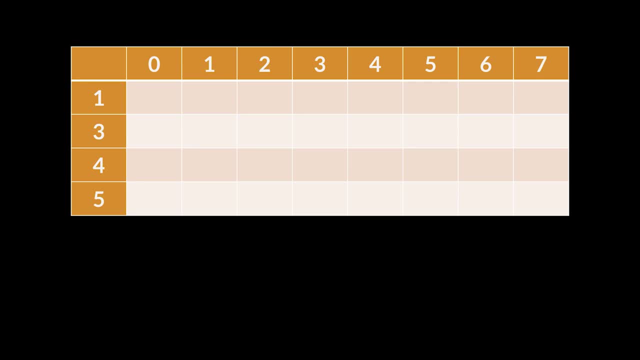 our sub-problems are the amounts taken individually, starting from 0 up until we reach the target value we want, which is 7 in this example. So in the first colon and first row, we are asking ourselves: what is the minimum number of coins required to produce the amount of? 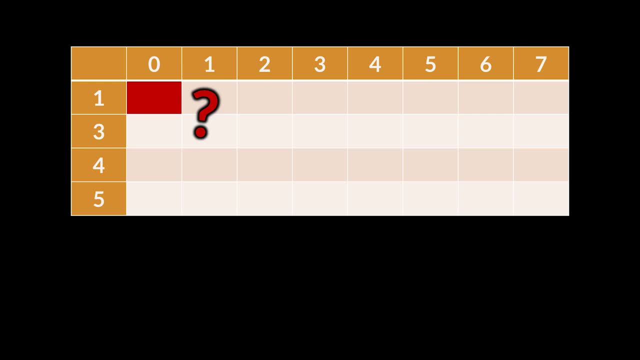 0,, given that we have an infinite supply of $1 coins only. Well, the answer is 0, no coins are required to do that right, And that remains true even after adding all the coins shown in that colon. Now, concerning the first row, all we have are $1 coins then to produce. 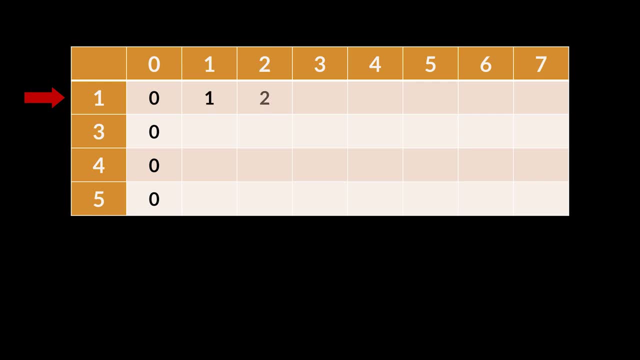 the amount of 1,, the minimum number of coins required is 1,, and to produce the amount of 2,, the minimum number of coins required is 2, and so on, right, All the way to the highest value, or 7,, which needs 7 $1 coins. Okay, concerning the following rows, the simple, 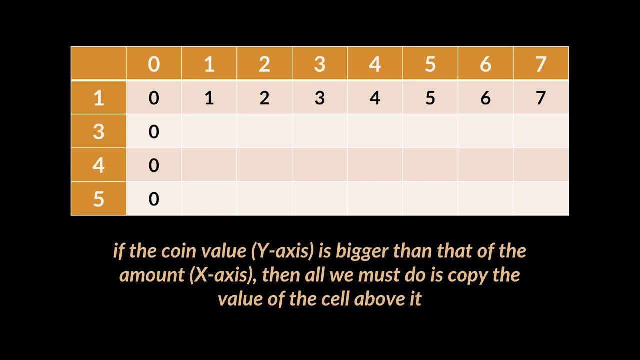 rule here is: If the coin value is bigger than that of the amount, then all we must do is copy the value of the cell above it. To explain this, take the next row where we added coin 3,, which means for the first colon. given an infinite supply of $1 and $3 coins, what is the minimum? 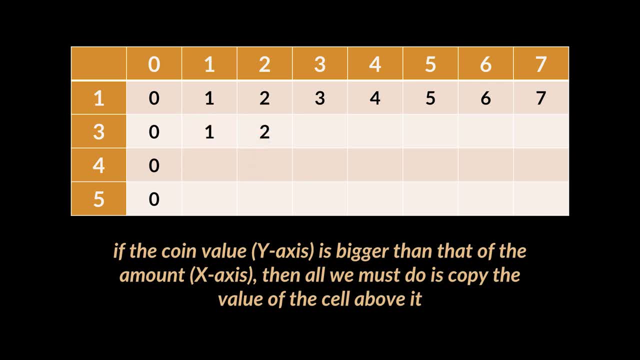 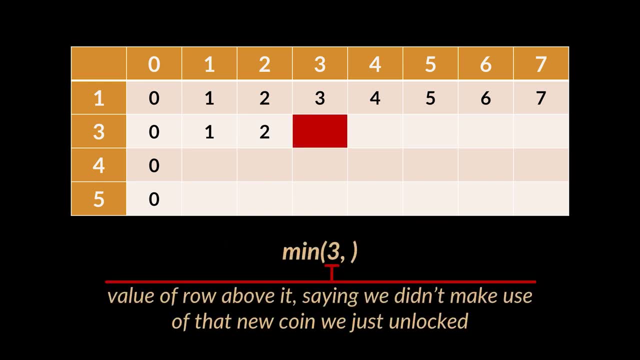 number of coins needed to make amount 1, and that is 1.. So we can copy the values of the row above it all the way until we reach the amount 3.. Now, at amount 3,, we need to pick the minimum between two values, the first one being the value in the row above it. basically, 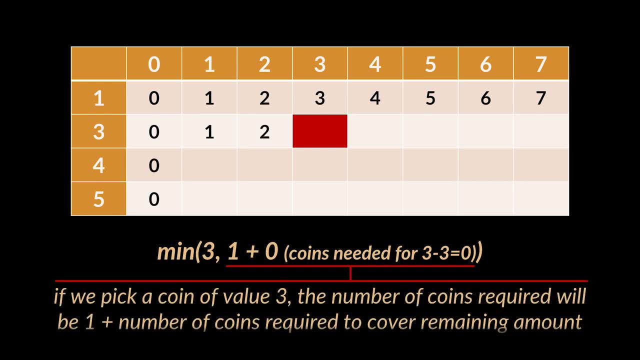 didn't pick a coin of value 3.. And the second one being: if we indeed pick a coin of value 3, then the number of coins required will be 1 plus the number of coins required to cover remaining amount, which is 3 minus 3 equals 0. So we hop to the zero amount in. 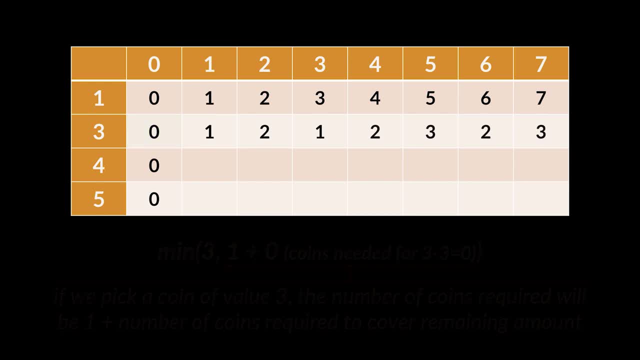 the same row and add that number to the 1.. Now, using the same approach, you can go ahead and fill the whole row right. For the following rows it is the same. we start by filling the same amount in the row above the one we are dealing with until we hit an equal or higher. 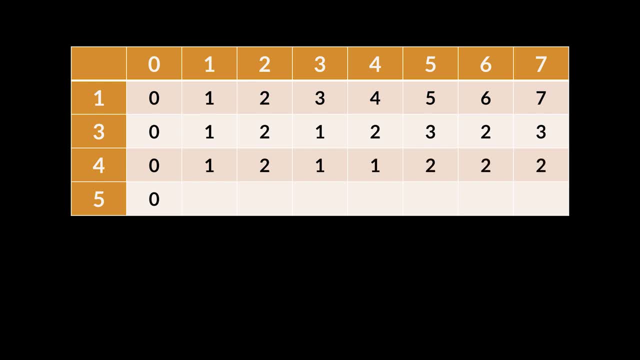 amount than the coin we just made. Alright, we are done, Let's start. See you in the next. we just unlocked. Then we apply the same minimum formula we just covered on the remaining columns. The last value we calculate, stored in the last row, last. 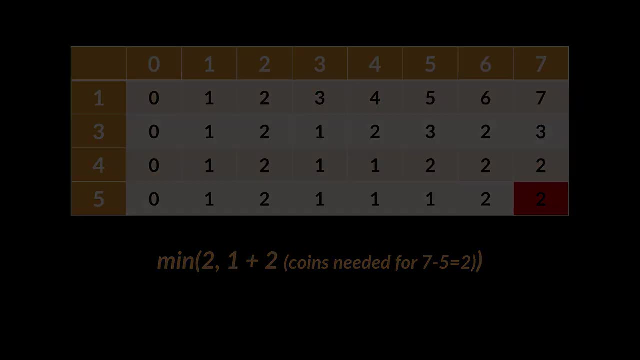 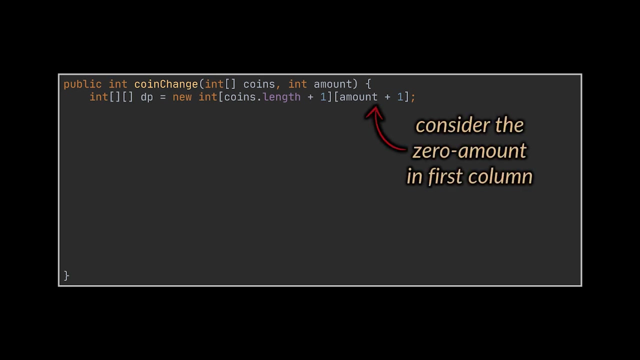 column will be the result we are looking for. To implement this, we are going to do exactly as we explained. We are going to start with a 2D array. We added an extra column to the amount because, if you recall, we also have the zero amount to. 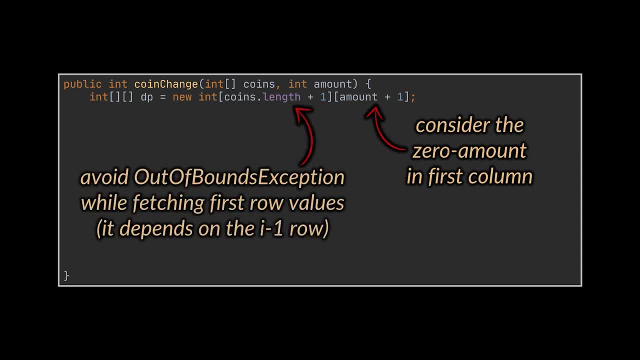 take into consideration, and we added an extra one for the coins, because each row depends on the one preceding it or above it. So if we were to apply the logic we discussed, as is on the first row, by fetching the i-1 row, it will throw. 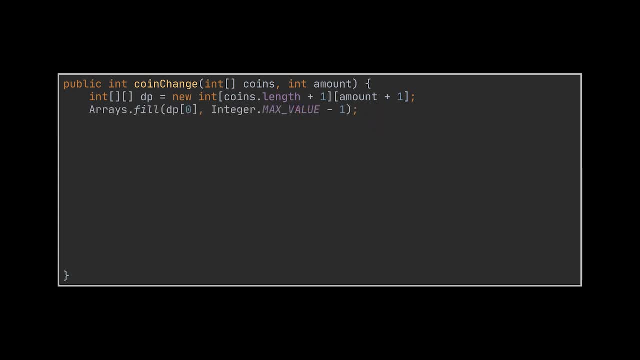 an out-of-bounds exception. So the first dummy row will be populated with the max integer value, as we will be performing the minimum operation using these cells. Then we will have our first loop that goes over the coins. This will simulate us adding one coin at a time. The first column will be populated with a zero, as 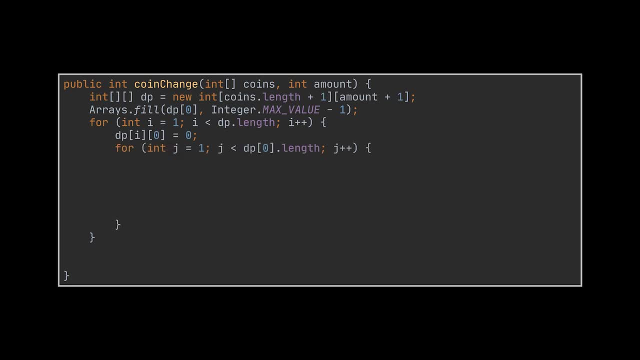 we mentioned, Then the core logic will sit inside a second loop that goes over the amounts, starting at value 1.. Here we will check: if the value of the coin is bigger than the amount, Then we copy the value from the row above it, and if not, we apply the formula. 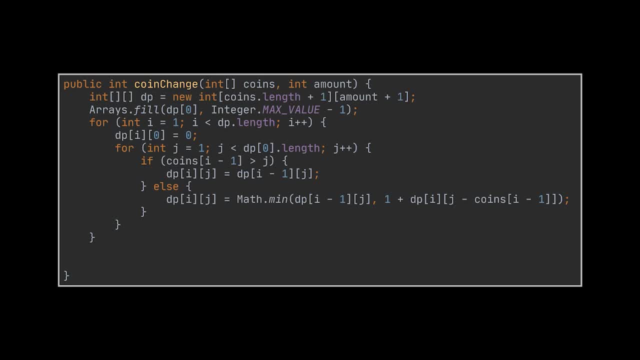 Meaning. we set the current value to be the minimum between the value above it and 1 plus the current amount minus the number of coins needed to fill the gap, which is located on the same row. We made use of i-1 instead of i in the